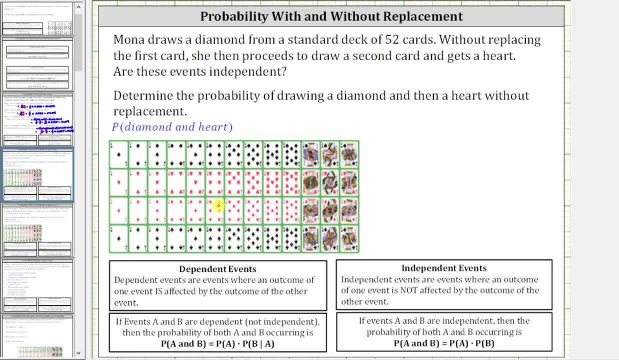 Mona draws a diamond from a standard deck of 52 cards, as shown here, Without replacing the first card. she then proceeds to draw a second card and gets a heart. Are these events independent? The two events are first selecting a diamond and the second event is selecting a heart. 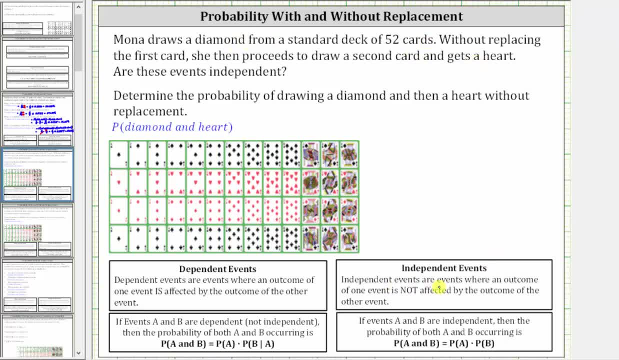 given a diamond was selected and not replaced. Remember, independent events are events where an outcome of one event is not affected by the outcome of the other, which, in this case, the outcome of selecting a heart is affected by the outcome of selecting a diamond. 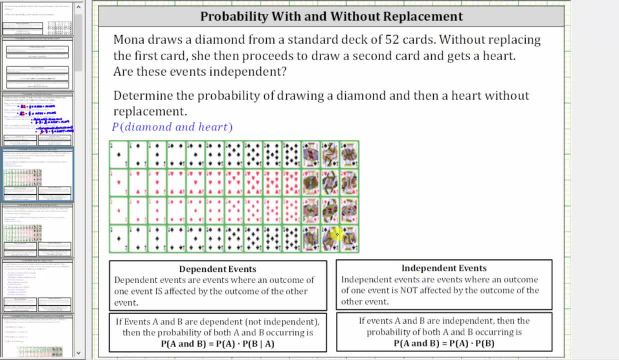 because the diamond was not replaced back into the deck And therefore these events are not independent. they're actually dependent, where dependent events are events where an outcome of one event is affected by the outcome of the other. So because Mona does not put the first card, 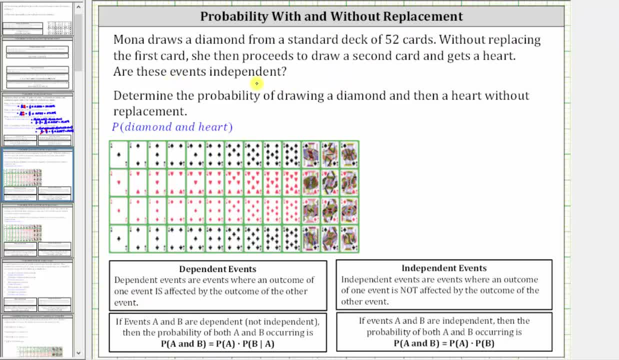 back into the deck. these two events are dependent, not independent. so we answer no, the events are not independent. And now we're asked to find the probability of drawing a diamond and then a heart without replacement. Because the two events are dependent, not independent. 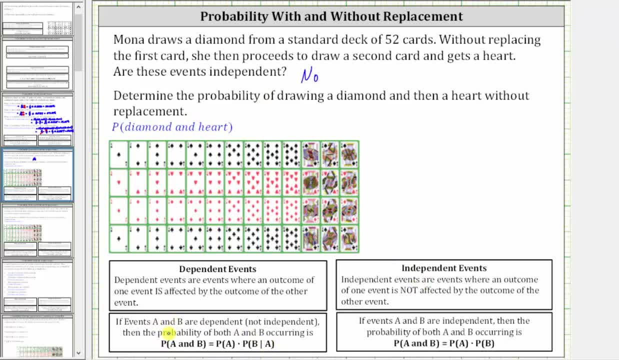 we find the probability using this formula here, where if events A and B are dependent, then the probability of both A and B occurring is equal to the probability of A. the first event times the probability of B, given event A has occurred. 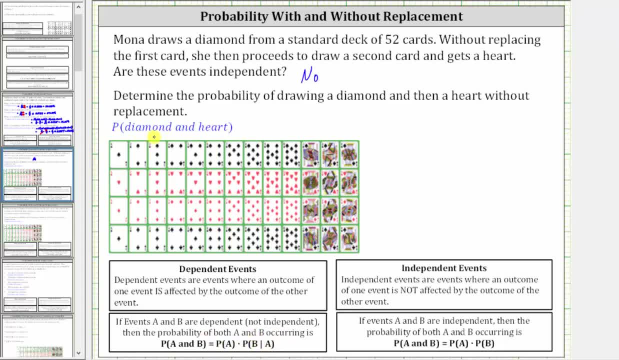 which we indicate using this notation here. So the probability of a diamond and a heart without replacement is equal to the probability of a diamond diamond times the probability of a heart given a diamond on the first card without replacement. So now let's find the probability of selecting a diamond. 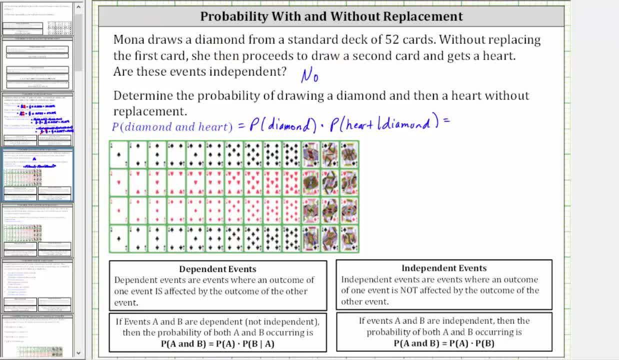 from a standard deck of 52 cards. Well, there are a total of 13 diamonds, so there are 13 favorable outcomes out of a total of 52 cards, or 52 possible outcomes, and therefore the probability of selecting a diamond is 13 divided by 52.. 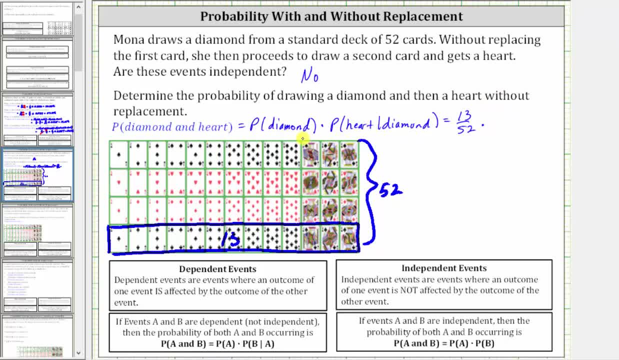 And now we need to find the probability of selecting a heart, given the diamond selected was not replaced. Let's just say the first card was the ace of diamonds here, and since it's not replaced, notice how now there are only 51 cards to select from. 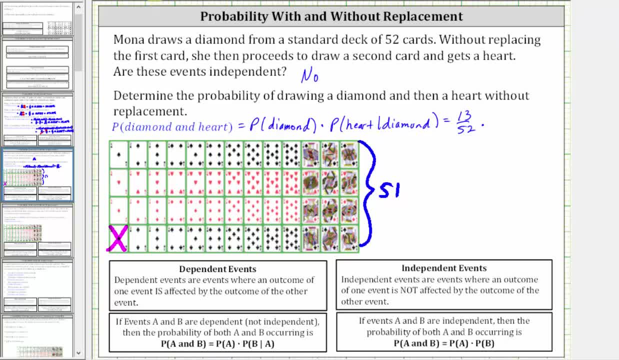 which is why the two events are dependent. of the 51 cards Notice, 13 of them are hearts. so now there are 13 favorable outcomes out of a total of 51 outcomes and therefore the probability of selecting a heart given. a diamond was selected and not replaced. 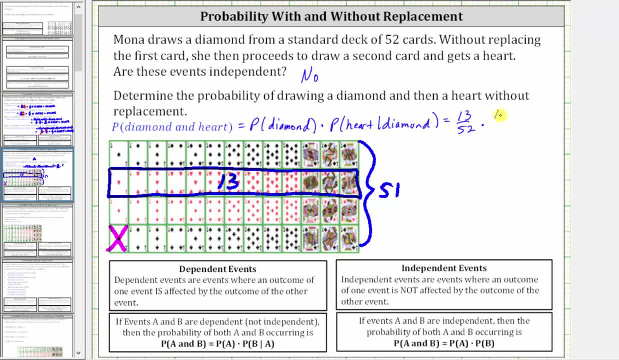 is 13 divided by 51. And we can simplify before multiplying. One way is to recognize that 13 52nds is equal to 1 4th. or we can recognize that 13 and 52 share a common factor of 13,, where there's one 13 in 13 and four 13s in 52.. 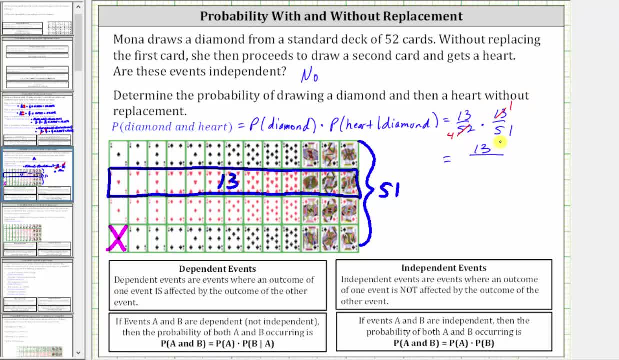 Multiplying: in the numerator, we have 13 times one, which is 13.. In the denominator, we have four times 51, which is 204.. So this is the probability of drawing a diamond and then a heart without replacement. but let's also convert to a decimal and a percentage. 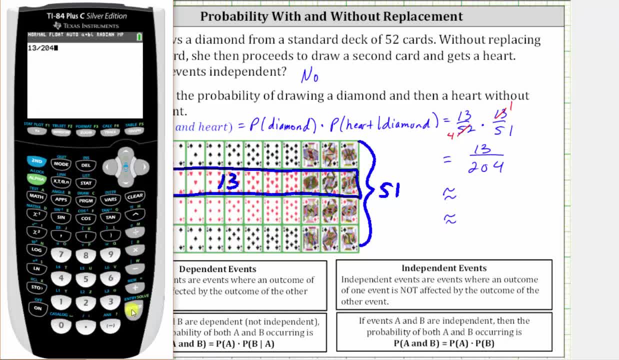 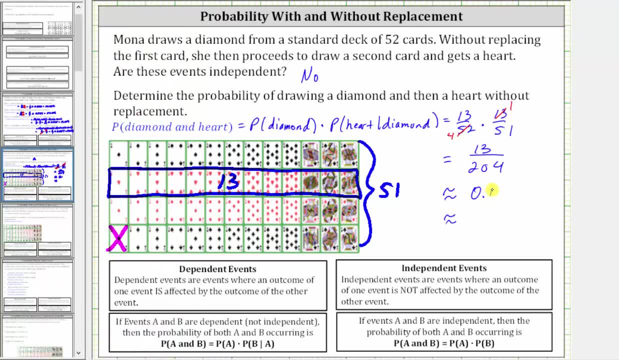 13 divided by 204. To four decimal places is approximately 0.0637,, which gives us approximately 6.37%. And now let's look at the situation again with replacement. Rhonda draws a diamond from a standard deck of cards. 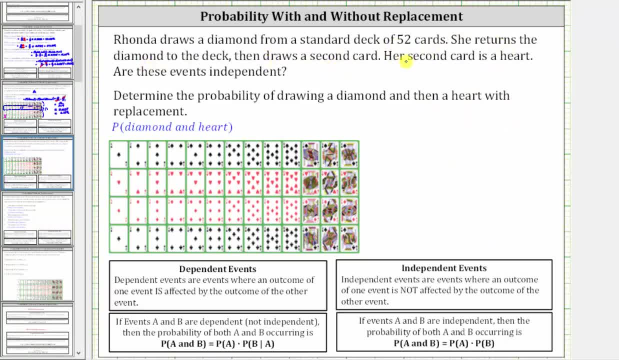 She returns the diamond to the deck and then draws a second card. Her second card is a heart. Are these events independent? So in this case, because she replaces the first card, which is a diamond, back into the deck, the outcome of the first event does not affect the outcome. 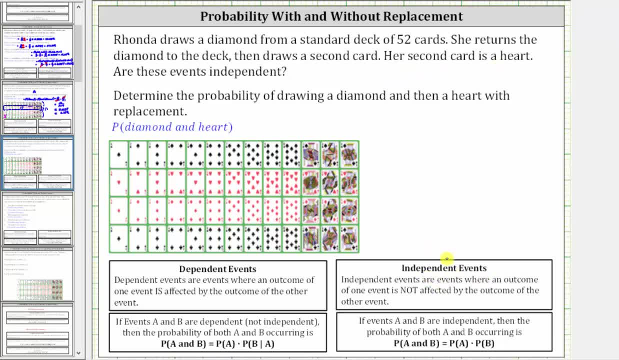 of the second event, of drawing a heart, and therefore the two events are independent. So we answer yes, the events are independent. And because the events are independent, we use this formula to find the probability that both occur, With the events A and B are independent. 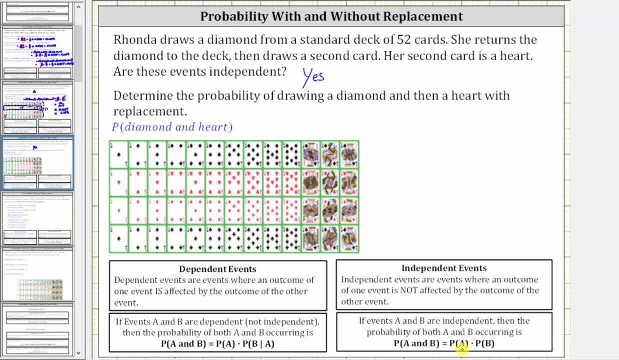 then the probability of both occurring is equal to the probability of A times the probability of B. So in this case, if we have replacement, the probability of a diamond and a heart is equal to the probability of a diamond times the probability of a heart.